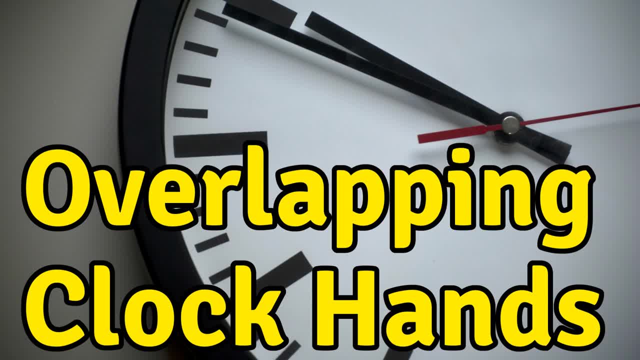 So you might know about the overlapping clock hands problem, which asks a very simple question: The minute hand and the hour hand of a clock are exactly overlapping. How much time is going to pass until they are exactly overlapping again? The answer to this problem, however. 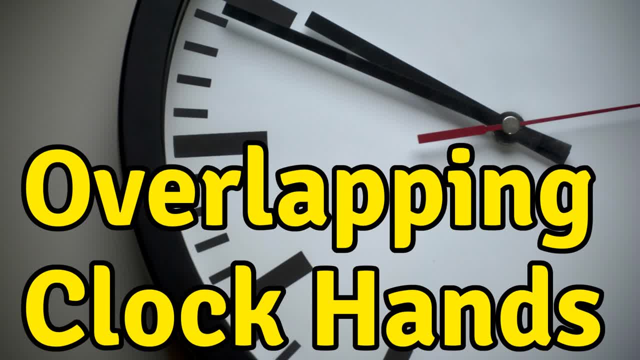 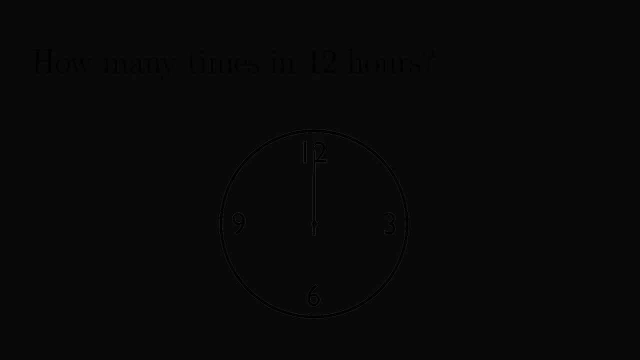 can be very simple to quite complicated, depending on your approach. I am going to present four different ways of solving the problem, and I'd like to start with the most elegant one. Alright, for our first method. we simply ask ourselves: how many times will the hands overlap? 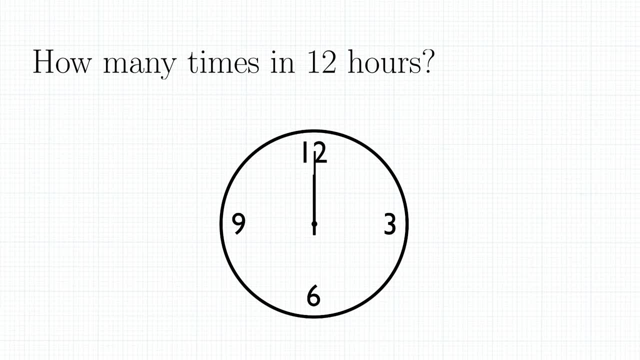 in a 12 hour interval. We will now start the clock and we will be able to count the overlaps. If you have a clock or watch in hand that you can manipulate, feel free to try this out for yourself. Okay, I counted 11 overlaps within 12 hours. 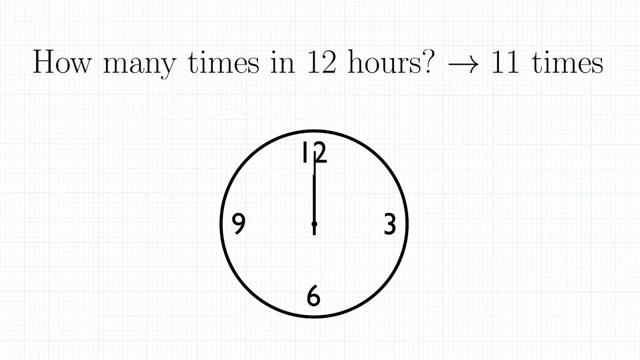 Note that when it's 12 hours, the clock will start to count. Okay, I counted 11 overlaps within 12 hours. Note that when it's 12 hours, the clock will start to count Again. we must not count that overlap if we already counted the overlap at 12 o'clock. 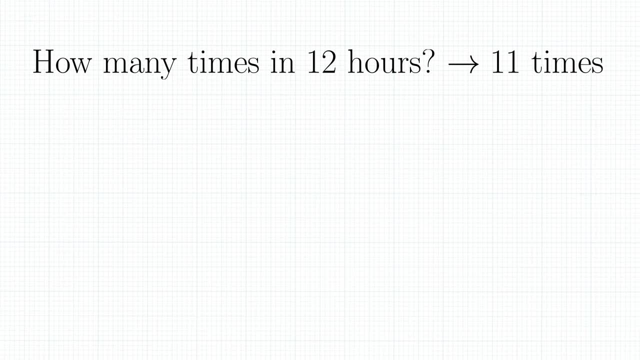 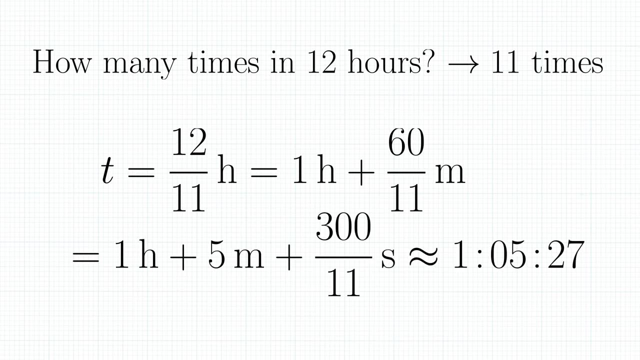 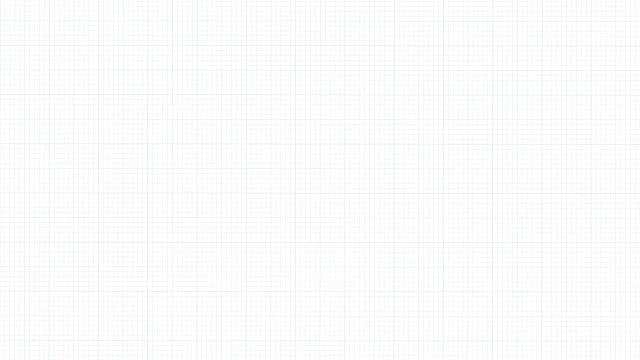 at the beginning. Since the 11 overlaps are evenly spaced, the time between two overlaps equals 12 over 11 hours, which is about 1 hour 5 minutes and 27 seconds. For the next methods, we need a way to measure the angle that the hands have moved since. 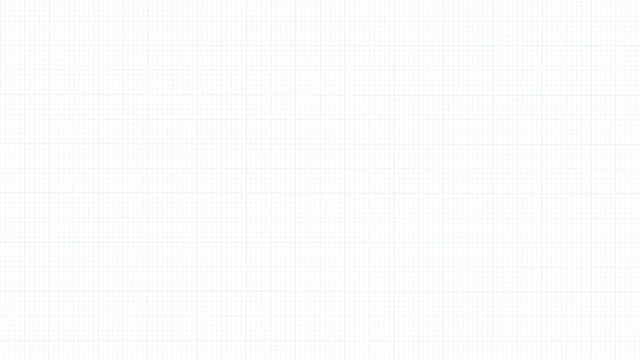 12 o'clock. I will use a system where one complete turn equals an angle of 1, half a turn equals an angle of 1, half a turn equals an angle of 1, half, and so on. This makes the following calculations most compact: 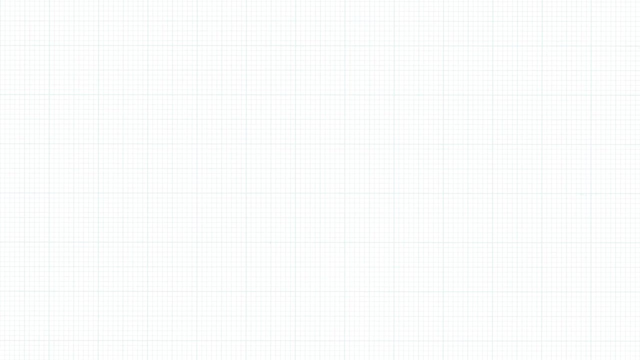 We can now introduce the angle that the hour hand has moved and I'll denote it by lowercase phi. Lowercase omega stands for the hour hand's angular speed. I do the same for the minute hand using uppercase letters and of course, the minute hand is 12 times as fast completing. 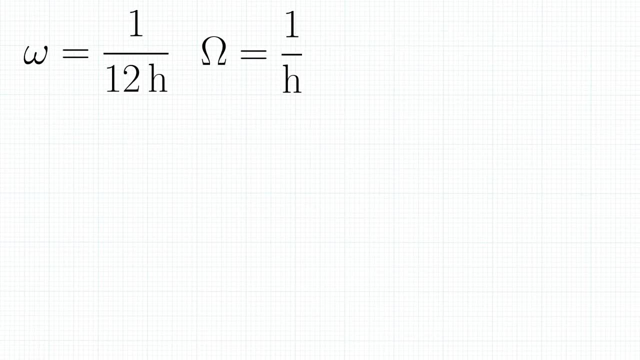 a turn in an hour. Now the second way to calculate the time between overlaps is to use the relative angular speed, delta, omega of the clock hands. They move apart at 11 over 12 per hour. Note that when they are a number of full turns apart, they are actually overlapping again. 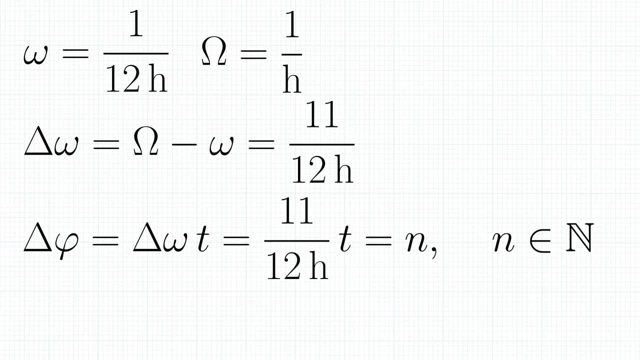 so we set the relative angle delta phi to any natural number To obtain the smallest non-zero interval. we set n to 1 and we find that t equals 12 over 11 hours again Okay. the third method is a little more brute force. 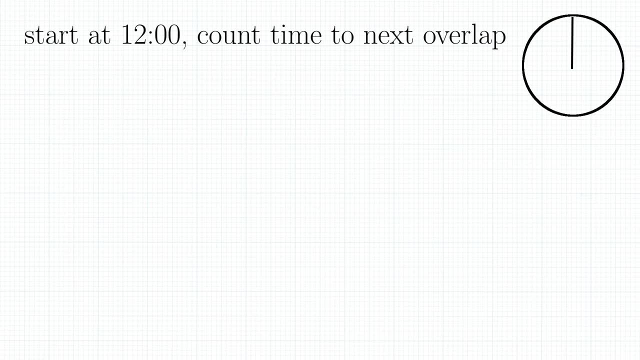 I remind you that the angle of the clock hand is the angle of the clock hand and the angle of the clock hand is the angle of the clock hand. Note that we imagine our clock starting at 12, and now we are going to count the time. 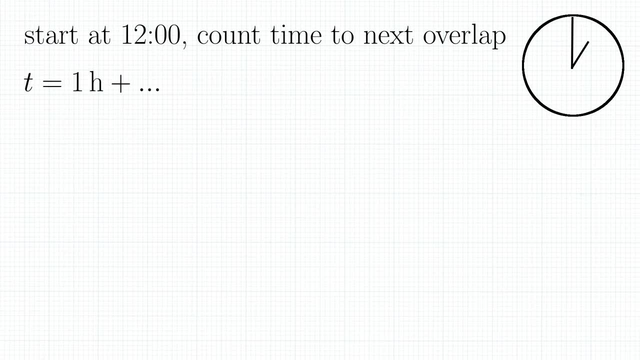 to the next overlap. Fast forward one hour and the minute hand will be at 12 again, while the hour hand has moved to 1.. We note that one hour has passed. Now the minute hand needs to catch up, so we allow it to move an angle of delta phi equal to 1 over 12 to get where. 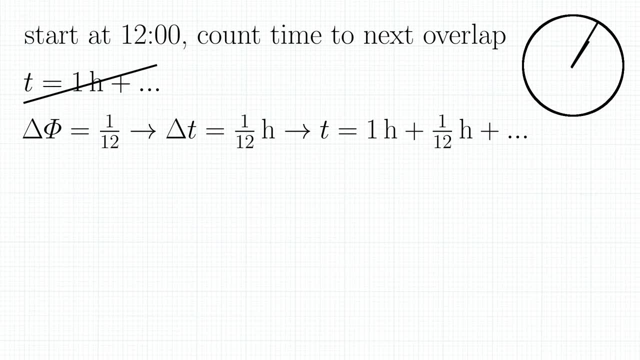 the hour hand currently is. This takes 1 over 12 hours, and we add that to our time total. The hands do not overlap, though, since they are a number of full turns apart, and they do not overlap since, meanwhile, the hour hand has moved a bit forward as well by delta. 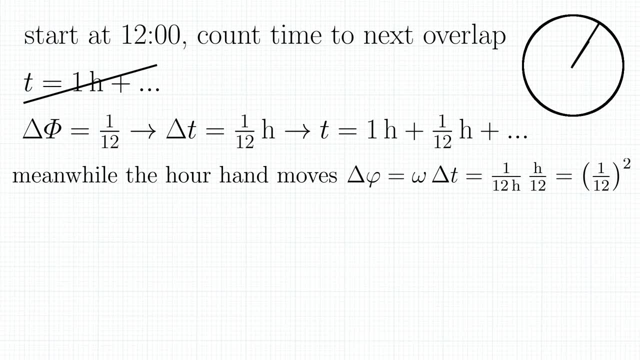 phi equals omega times delta t, which is 1 over 12 squared. Now, in order to catch up, the minute hand has to travel. this additional angle which takes delta t equals delta phi over omega equals 1 over 12 squared hours. So we add: 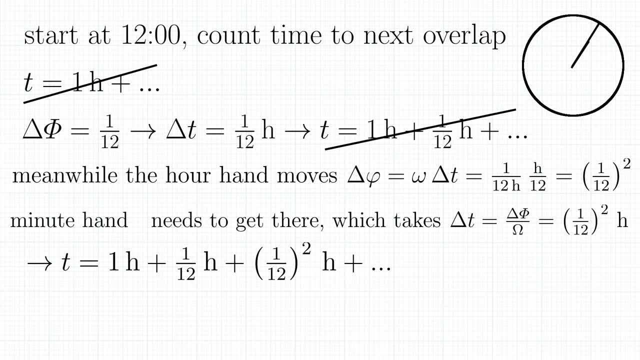 that to our time total and we start to see a pattern. If we were to go through another iteration of this, we would find a term with a power of 3, and so on. We can therefore write the time as an infinite series. 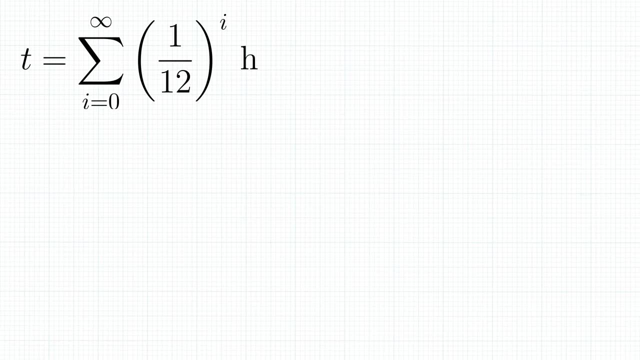 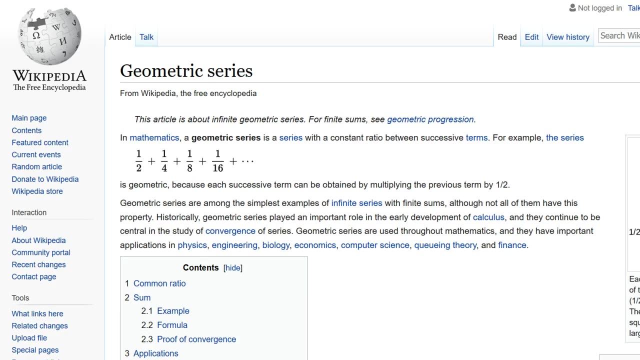 If we did everything correctly. this series needs to converge, since the clock hands do overlap in a finite amount of time, And in fact it does. It is a simple case of the geometric series and there is a formula for it. This is the most general expression and it is. 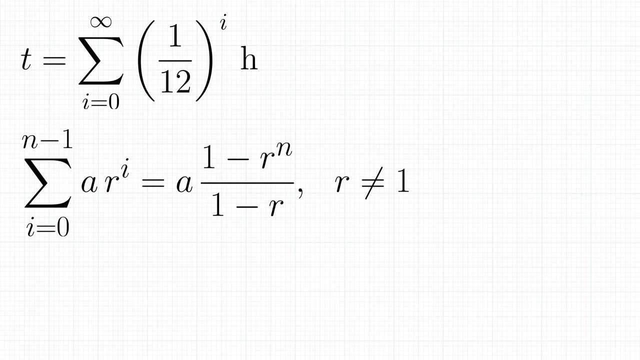 true for any r that isn't 1.. Now, in our case, a is 1, r is 1 over 12, and n equals infinity. Since r is smaller than 1, r to the power, n vanishes as n goes to infinity. 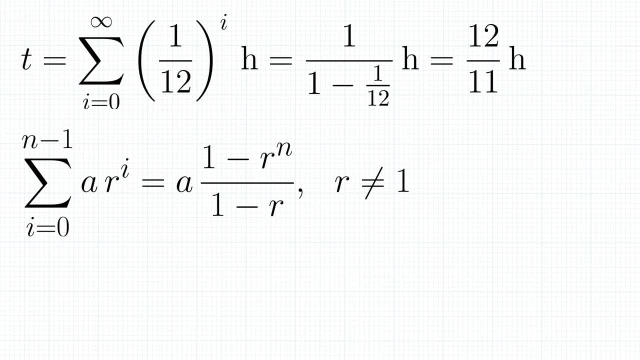 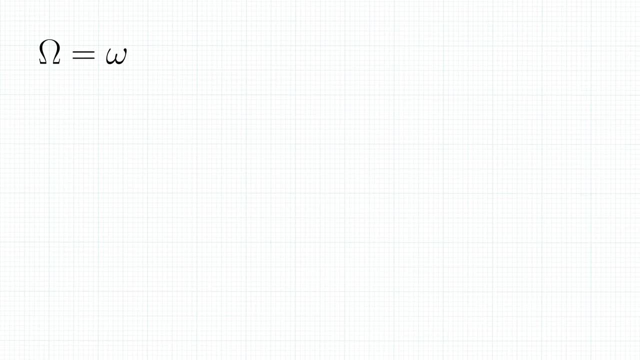 and we are left with 1 over 1 minus 1 over 12 hours, which is exactly 12 over 11 hours. again For the fourth method, we simply state that the angle travelled by both hands has to be the same for them to overlap. I think this is actually the most intuitive approach, but 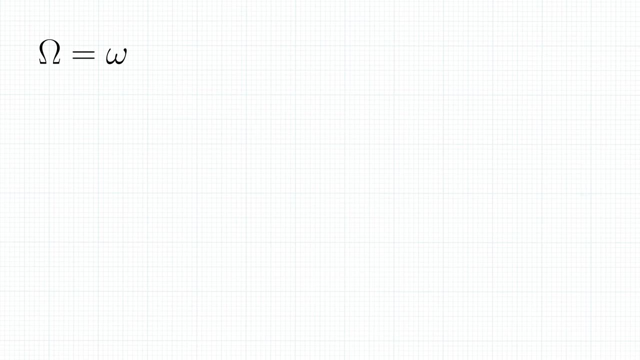 I also think it is the worst way of solving the problem. Anyway, It yields an equation for t that seems contradictory at first: t over 12 hours equals t over 1 hour. There is no contradiction, however, if we look at how the angle works for values. 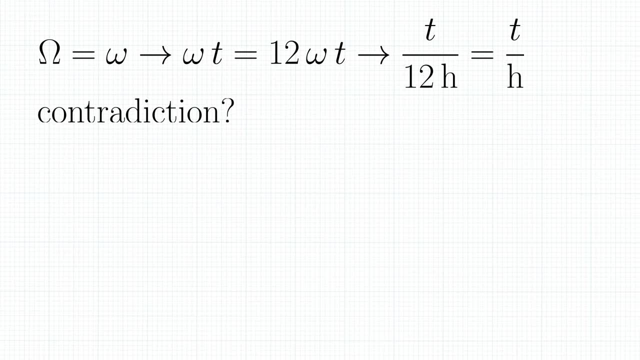 greater than 1.. 1 and a half turns, for instance, are equal to a half turn, and so are 2 and a half turns, and 3 and a quarter turns are actually just a quarter turn. For our equation to reflect that property, we need to apply a function on both sides that satisfies a. 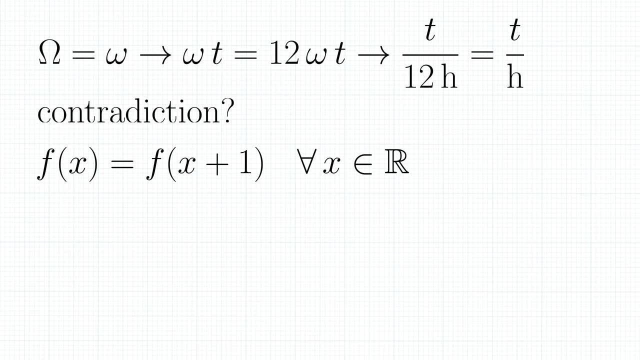 function: m onto t is 0 and x is 0 and t onto t is 1 and a half is 0 and a half. In the case of t over 12 hours, we apply the same function, the function on both sides. 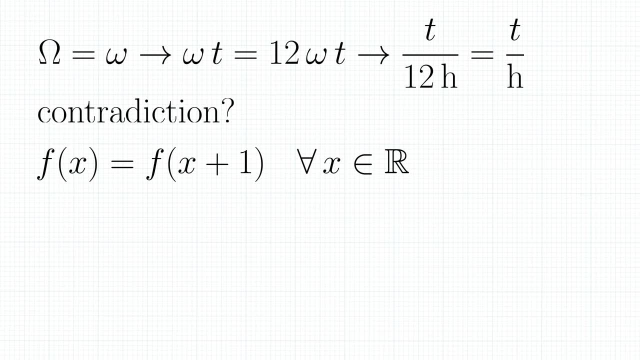 equals 1 by 0. We want to write that function as t over 12 hours. For the second approach, we simply enter: f of x is f of x plus 1.. A periodic function with period 1.. We are not limited to a period of 1, however, since we can just multiply the equation by. 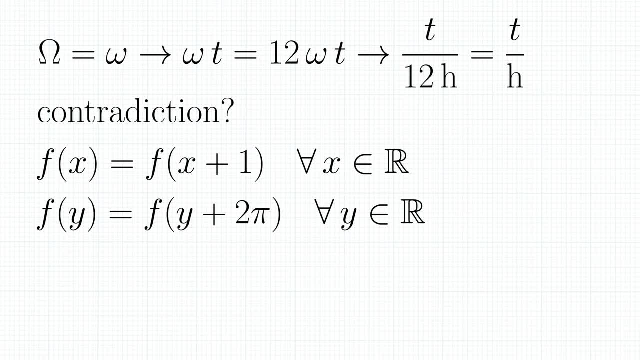 any constant and apply a periodic function where period equals that constant. The obvious choice here is 2pi, and the functions we are going to use are a sine and cosine function. You can think of the effect the periodic function produces as if we took the number ray cut. 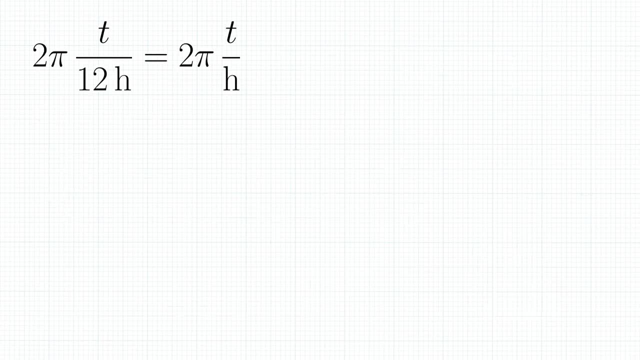 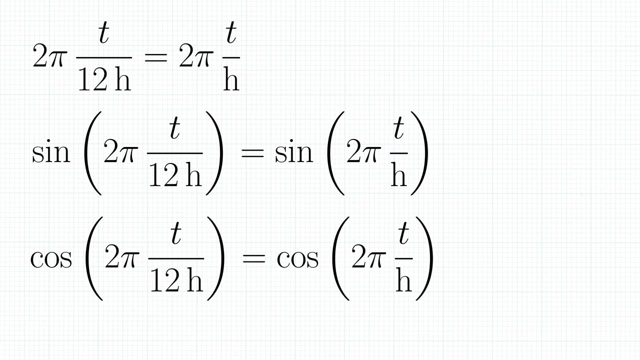 it off at 2pi and formed a circle out. Thank you of it. So we have our equation multiplied by 2pi and we are going to apply the sine function to both sides and the cosine function to both sides. We can now plug these equations into a computer algebra system to obtain numerical solutions. 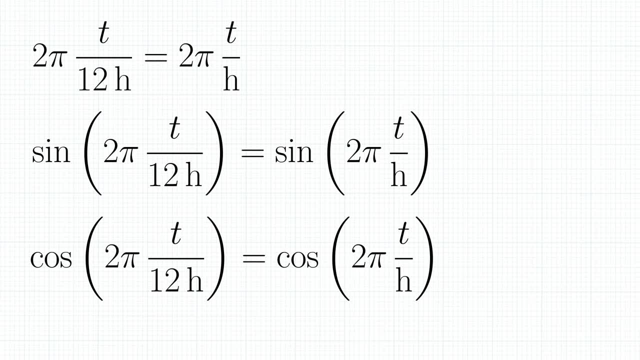 We are looking for the smallest non-zero value of t that satisfies both equations. If we only look at one equation, we get solutions to the equation that are no solution to the clock hands problem, and I think this is because sine and cosine are not only periodic, but